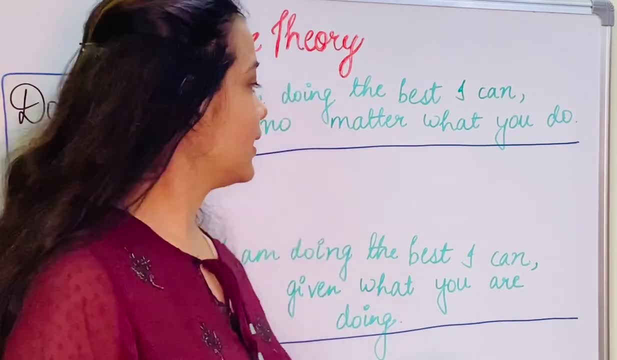 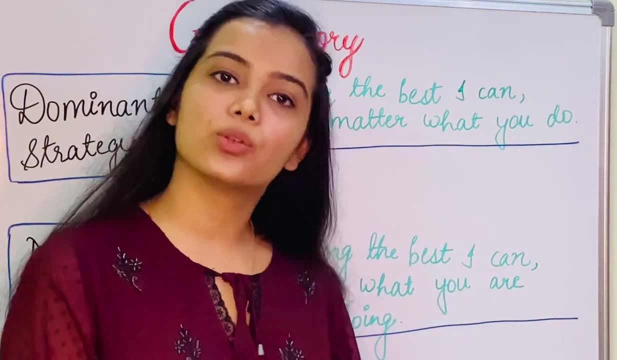 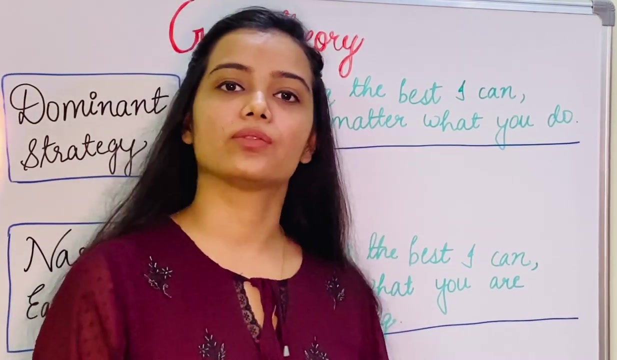 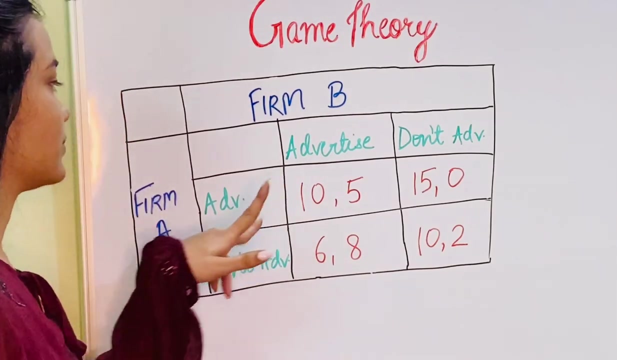 what I do, Whereas, on the other hand, Nash equilibrium is: I am doing the best I can, given what you are doing, or you are doing the best I can, given what I am doing. Now let's understand these concepts with the help of some examples. So here we have two firms, firm A and firm 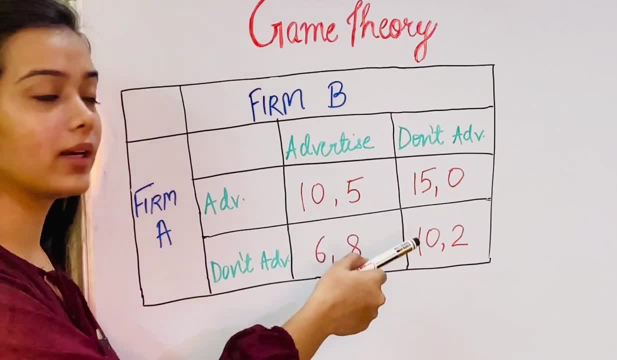 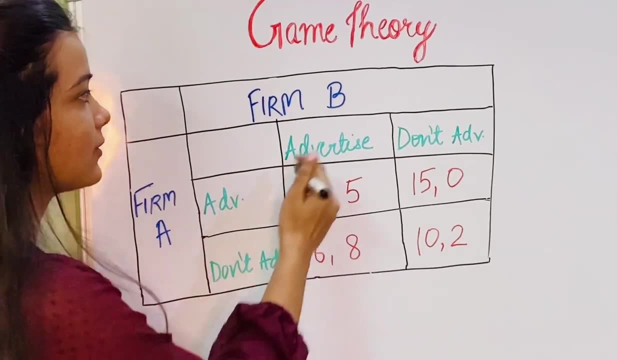 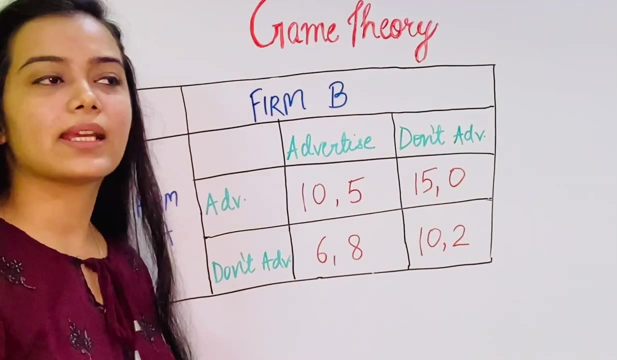 B and they have two options: either to advertise their product or not to advertise their product. So if we see firm A, if firm A also advertises and firm B also advertises, The payoffs are 10 and 5.. Now, what is a payoff? Payoff is any value associated with a possible 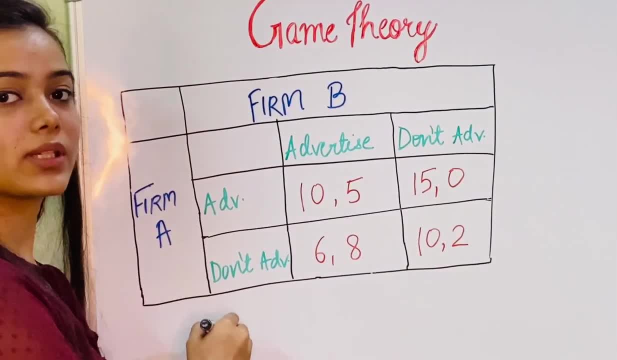 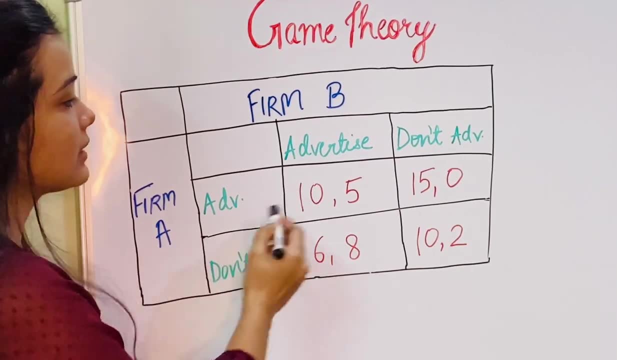 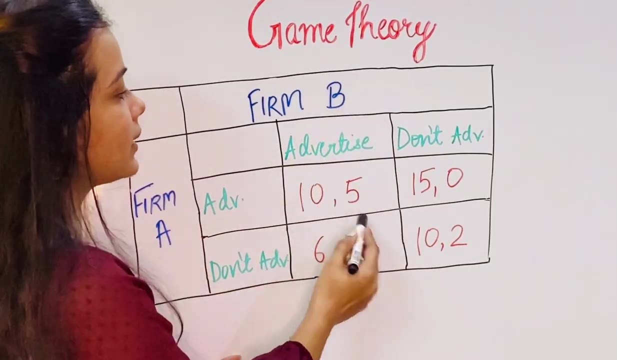 outcome, That is, if firm A also chooses to advertise and firm B also chooses to advertise, the payoff to firm A, that is, firm A will get a reward or will get a profit of 10, while firm B will get a profit of 5.. 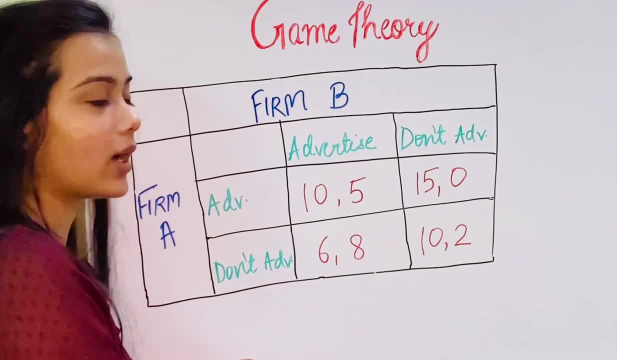 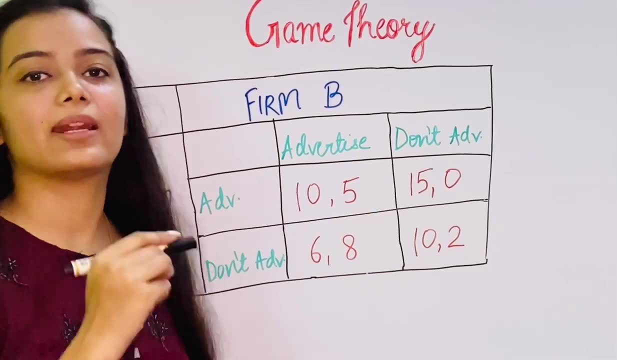 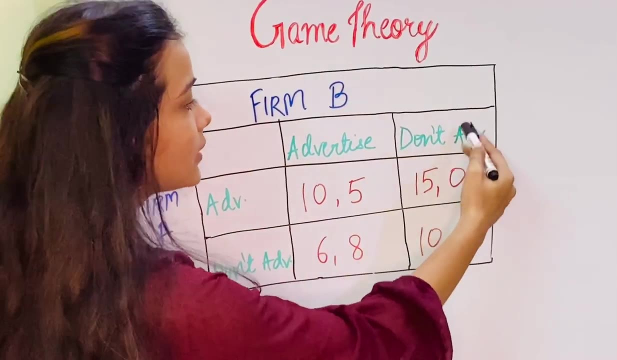 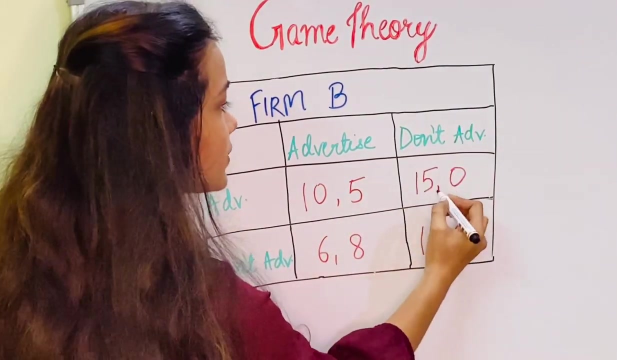 Now, all of these firms choose to advertise their product and they get the payoffs 10 and 5 respectively, provided that both of them are advertising. Similarly, if we see, if firm A advertises and firm B is not advertising, then the payoffs are 15 and 0.. 15 is the payoff. 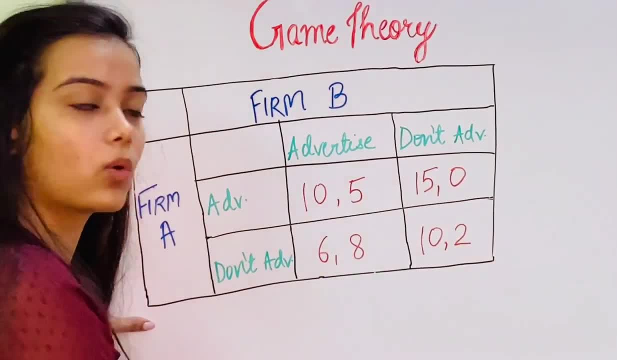 or 15 is the reward to firm A is advertising. So that's Bueno. and there is a point where if firm A and firm B are advertising, and guess what, if 16 is the payoff, Then we will get the yards each in this case, So that that is what we will see as the payoff, But if firm Bındaki 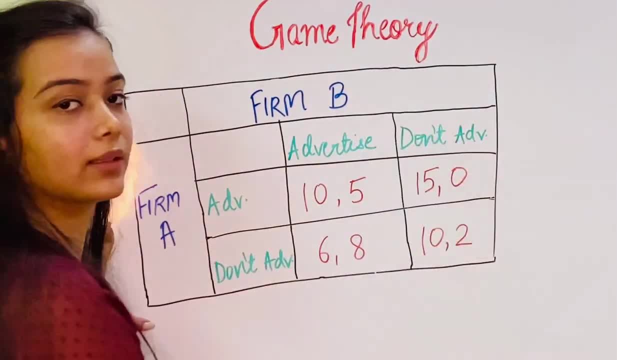 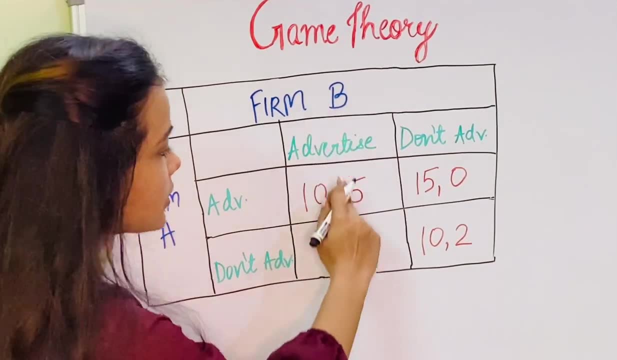 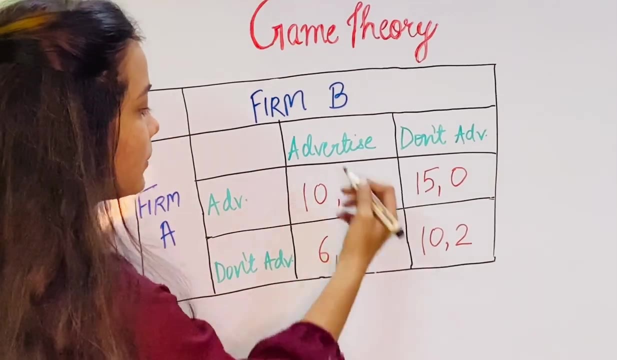 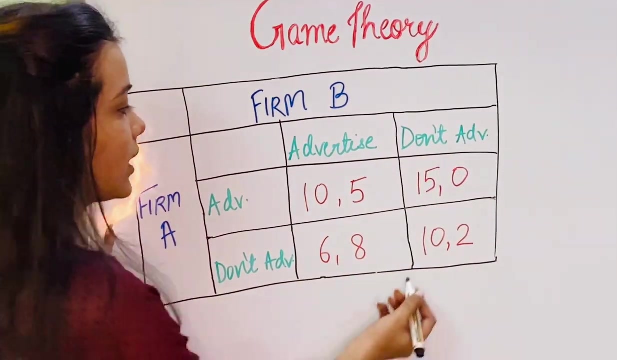 form A and 0 is the reward to form B. Similarly, we can see that if form A chooses not to advertise and form B chooses to advertise, so we have the reward. the payoff to form A is 6 and the payoff to form B is 8.. And if both of them choose not to advertise their product. 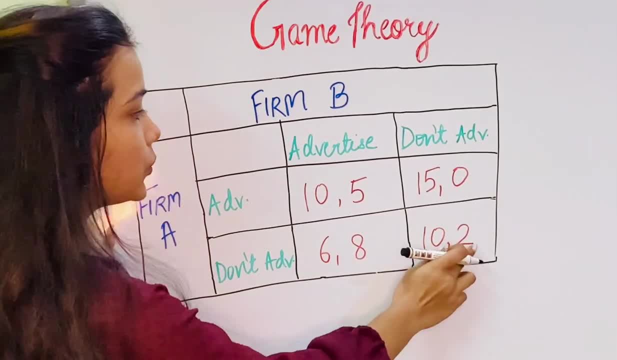 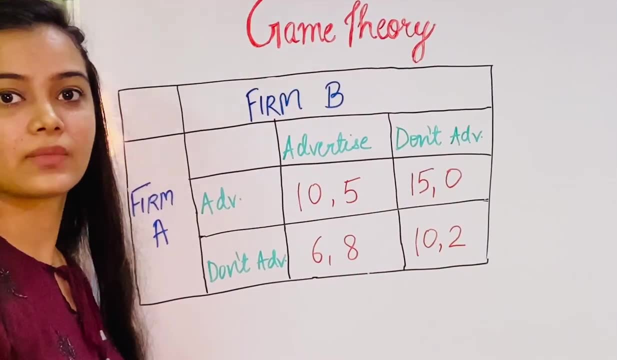 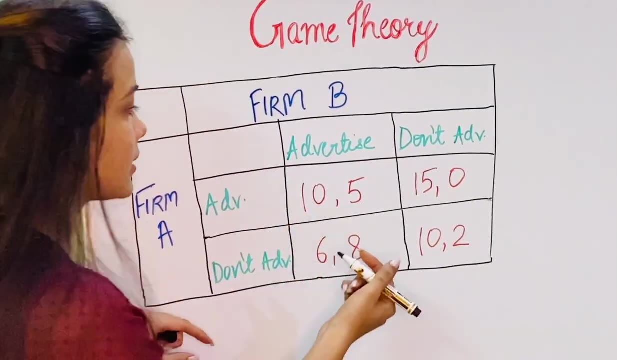 then 10 is the reward that goes to form A, and 2 is the reward that goes to form B. Now the question is which of these forms have a dominant strategy? For that, we need to consider their payoffs. Now. if we consider form A first of all, what are the payoffs? 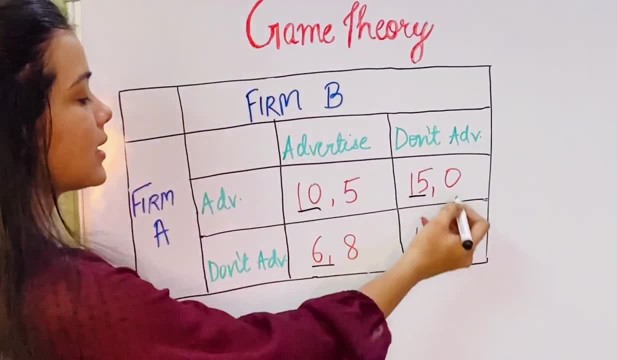 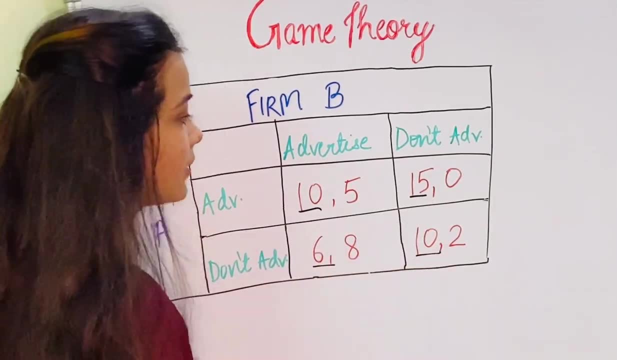 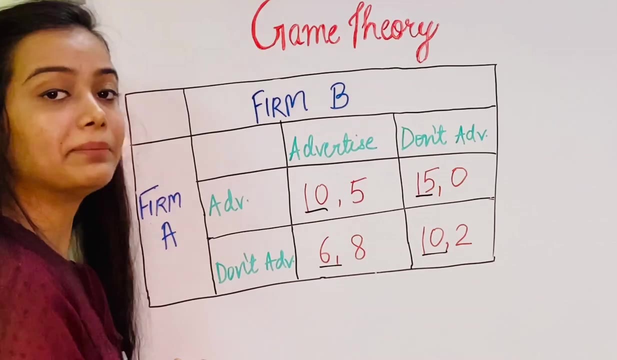 of form A. These: These are the payoffs that belong to form A, That is, 10, 15,, 6 and 10, all before the comma And all after the comma. these values are the payoffs that goes to form B. So here, while checking whether form A has a dominant strategy, 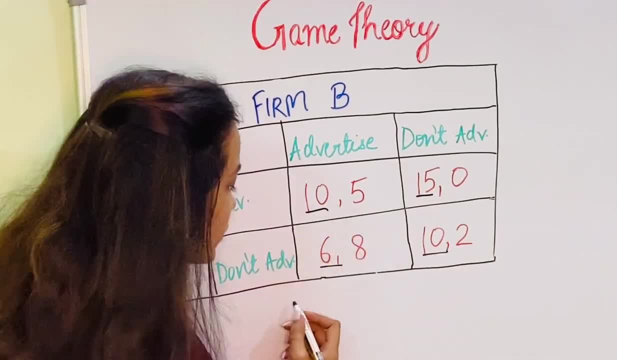 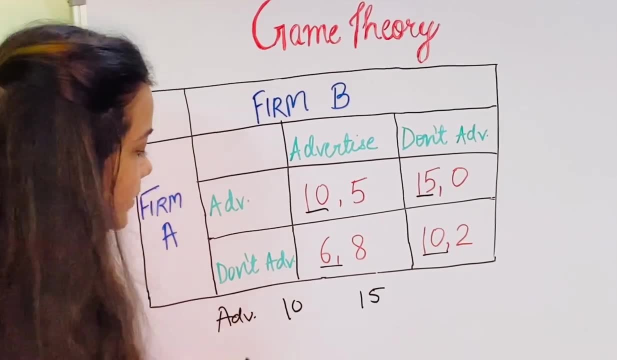 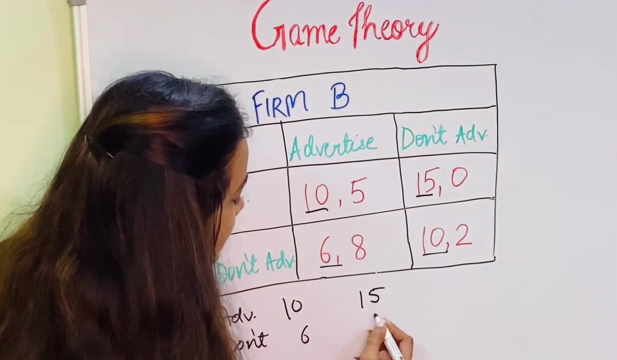 or not, we need to consider its payoffs. So here, 10 and 15,. these are the payoffs when the firm chooses to advertise, when form A chooses to advertise, And when form A chooses not to advertise, the payoffs are 6 and 10.. 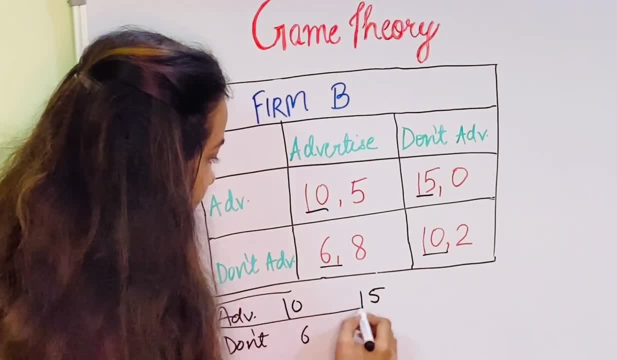 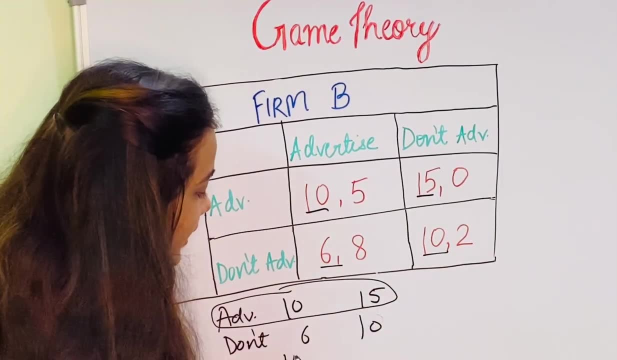 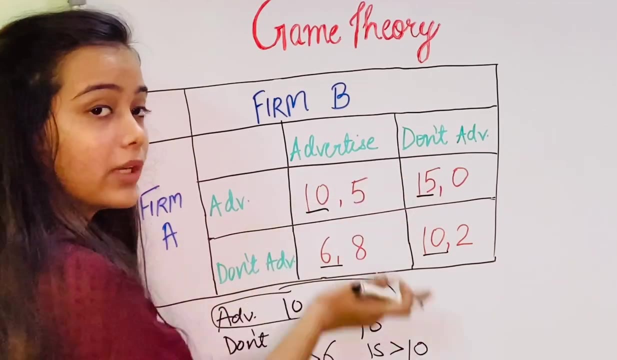 Clearly we can see that 10 and 15 are greater than 6 and 10 respectively, which means 10 is greater than 6 and 15 is greater than 10.. That means advertising. the payoffs that belong to advertisingmekaclub are greater than 2 times bigger than 5.. So these are the payoffs. 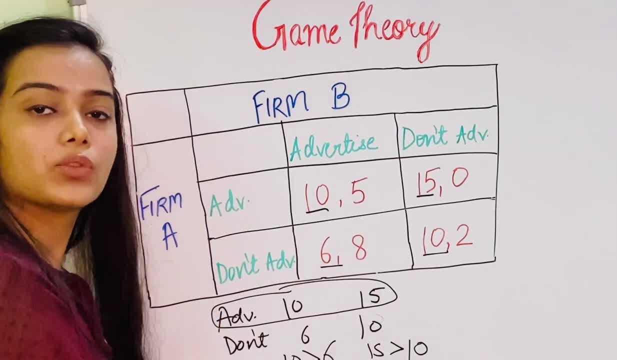 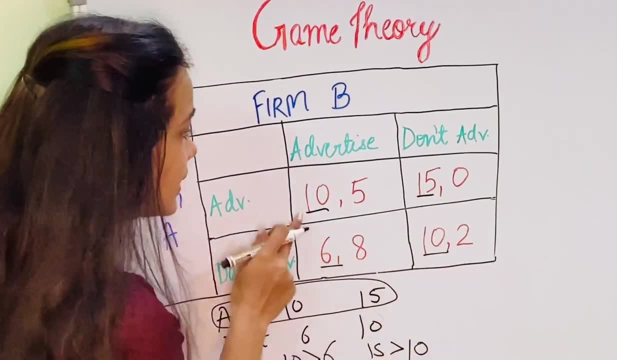 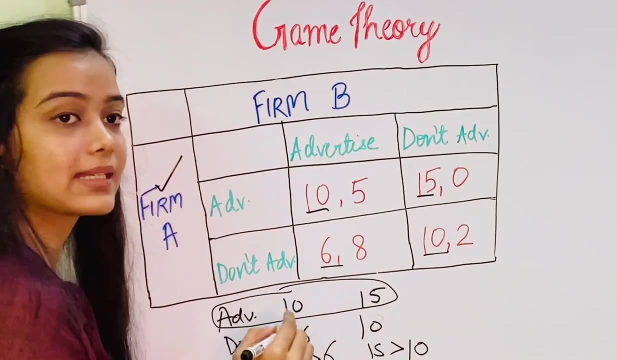 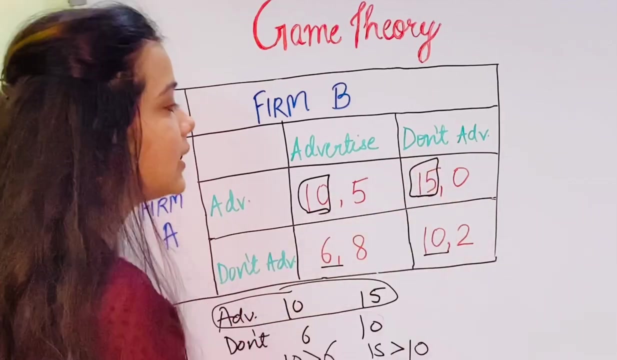 advertising that the firm A gets when it chooses to advertise are greater than when it chooses not to advertise, and both of them we can see 10 is greater than 6,, 15 is greater than 10.. That means firm A has a dominant strategy in advertising because both 10 and 15 are. 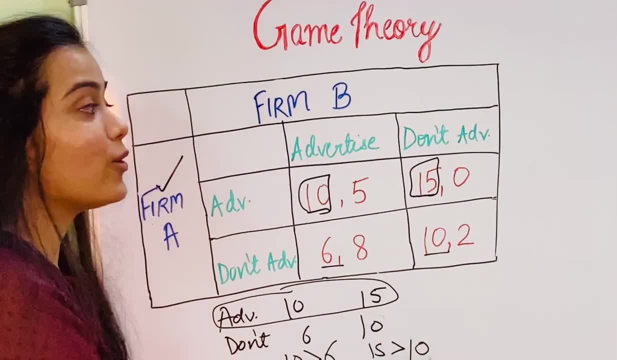 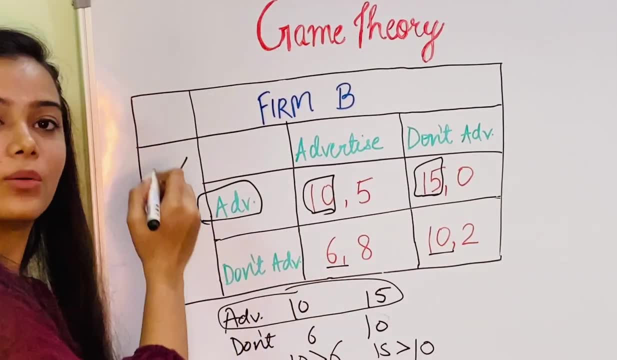 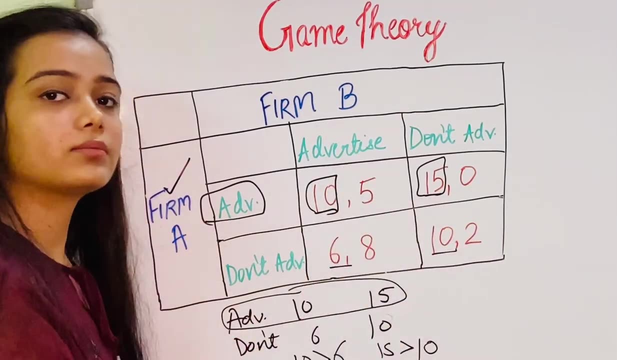 greater than 6 and 10 respectively. And no matter whatever firm B chooses, firm A will always choose to advertise because firm A has a dominant strategy in advertising. Now let's check whether firm B also has a dominant strategy or not. So, considering the payoffs, first of all, we have to 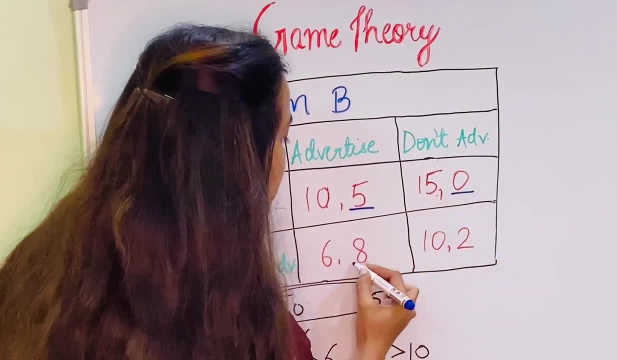 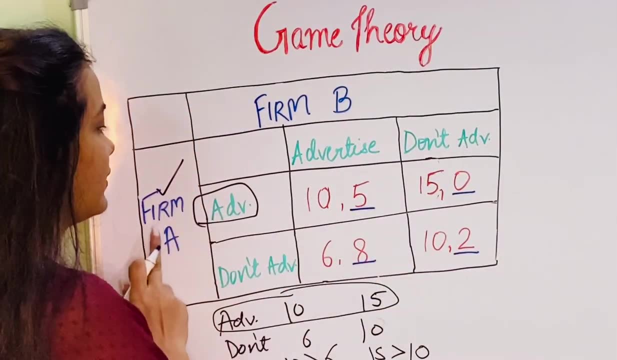 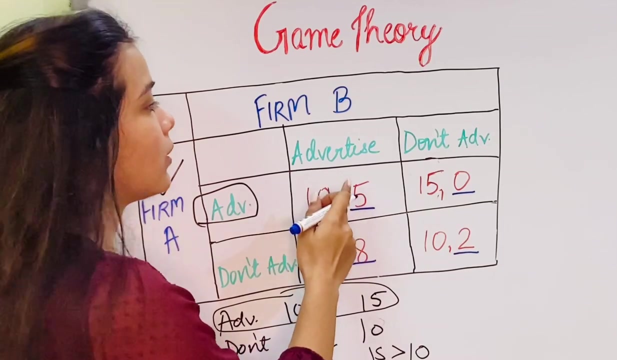 consider the payoffs of firm B, So all the payoffs after the comma. these belong to firm B. We have 5,, 0,, 8 and 2. That is, when firm A chooses to advertise and firm B also chooses to advertise, then 5 is the payoff or 5 is the reward that goes to firm B and similarly all the other. 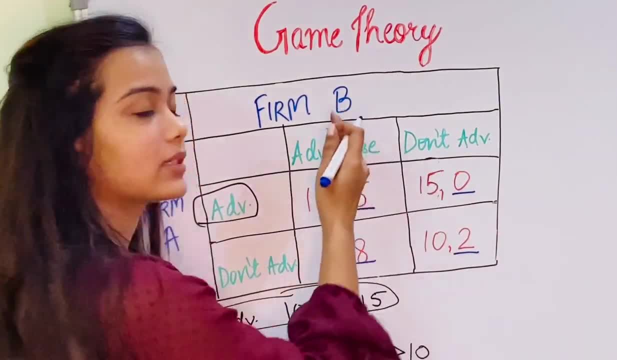 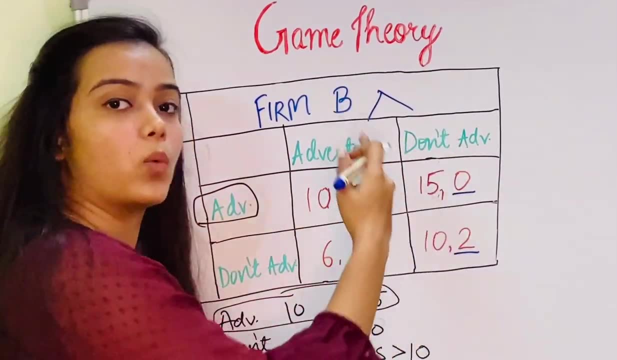 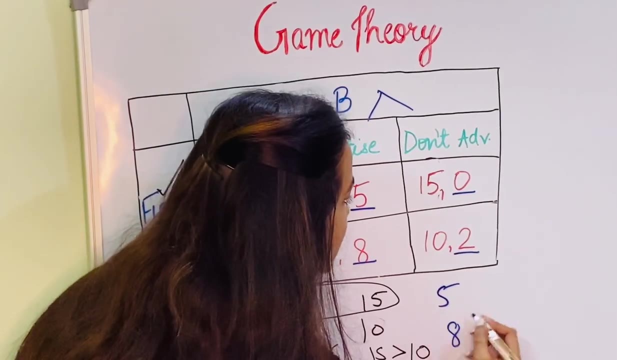 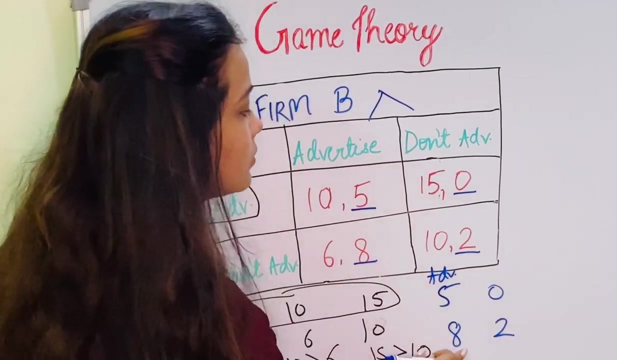 cases. Now we have to check whether firm B has a dominant strategy For that we know. now the options are this way, that is, the options are now vertically, So we have to check. then vertically, that is 5, 8,, 0 and 2, and so 5 and 8 belongs to advertising. These are the 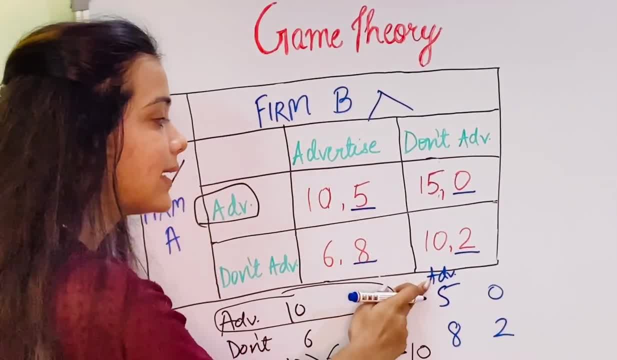 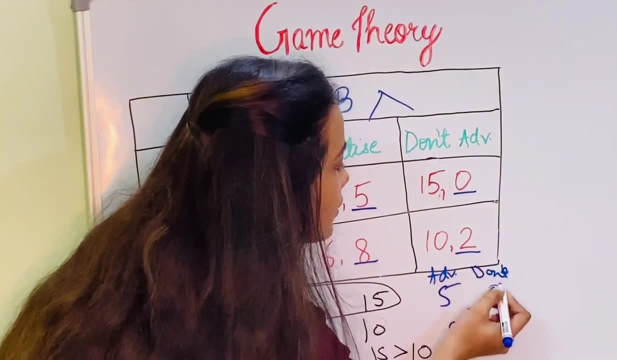 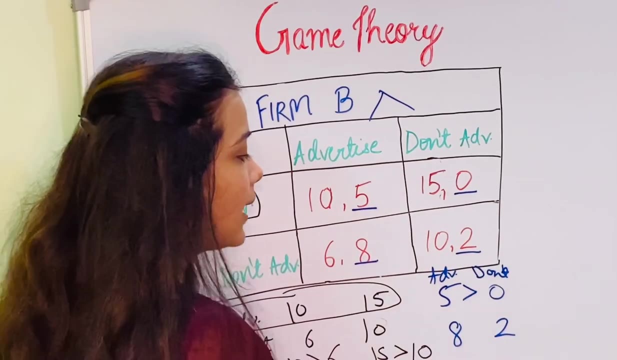 payoffs that belongs to advertising or that the firm gets these payoffs when the firm chooses to advertise and these payoffs when the firm chooses not to advertise. Clearly we can see that 5 is greater than 0 and 5 is the reward that goes to firm B. So we can see that 5 is greater than 0 and. 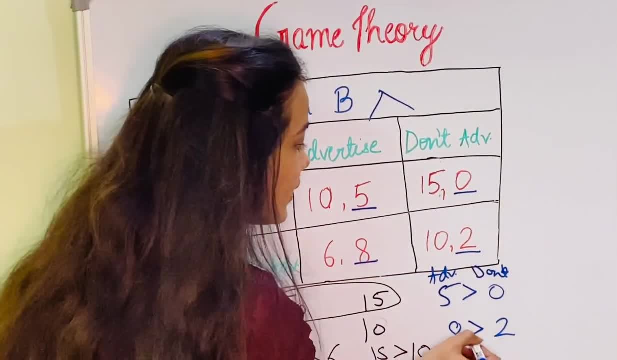 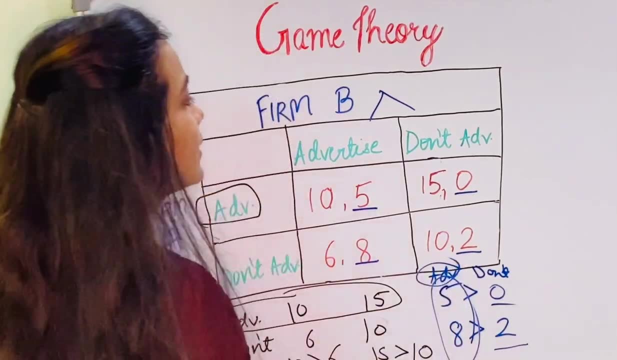 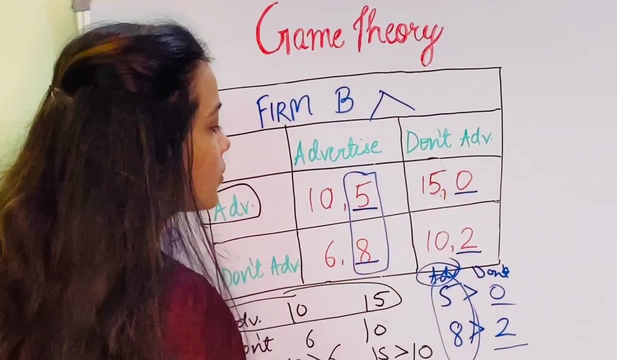 8 is greater than 2.. That means again, both of these are greater than both of these respectively. That means again, firm B has a dominant strategy in advertising because 5 is greater than 0 and 8 is greater than 2.. Now here we are looking vertically and not 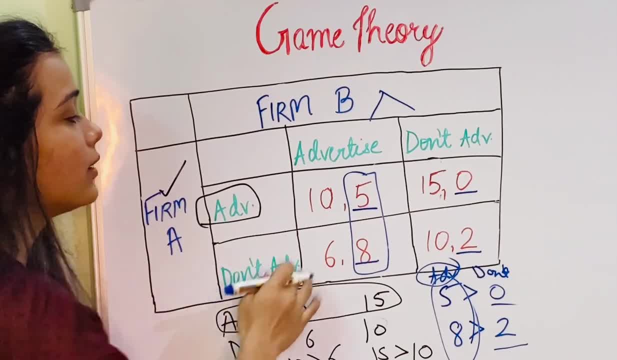 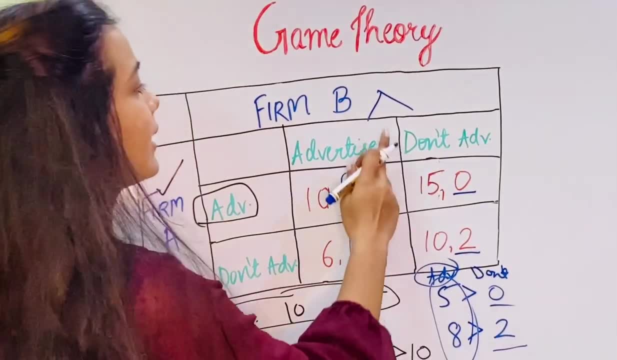 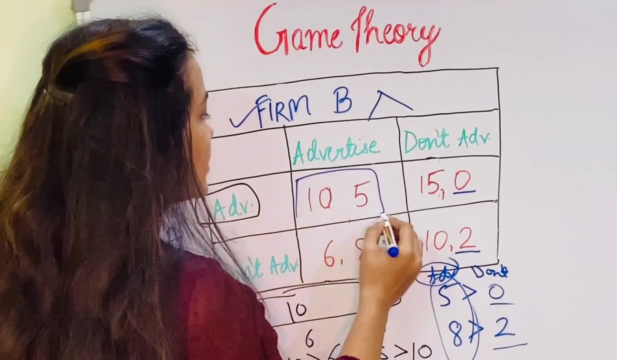 horizontally, while on the other hand, for form A, we looked horizontally. So after all of this, we can clearly say that firm B also has a dominant strategy in advertising. So now, if we see both of these have a dominant strategy in advertising, Now, considering that they, 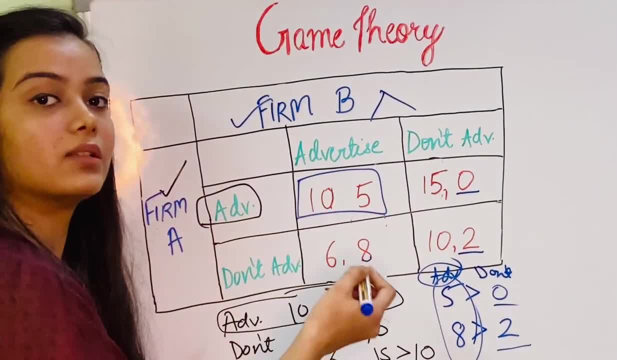 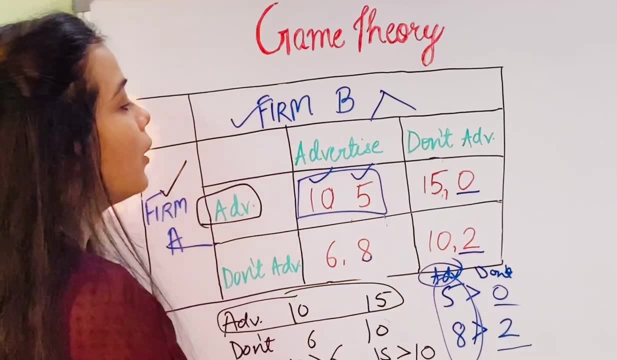 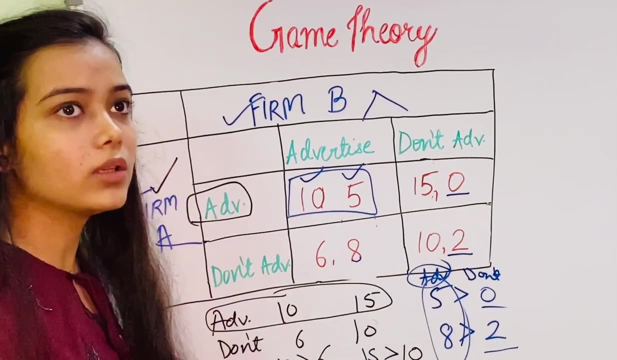 are rational, both of these firms will choose to advertise, and firm A will get a payoff of 10 and firm B will get a payoff of 5.. Now let's consider a slightly different example, wherein because we know that not all the games have dominant strategies for each player. Now let us consider 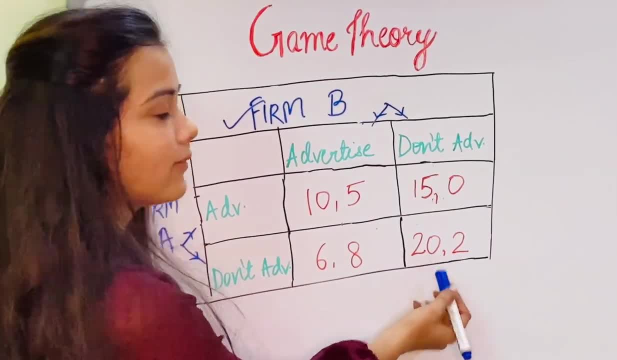 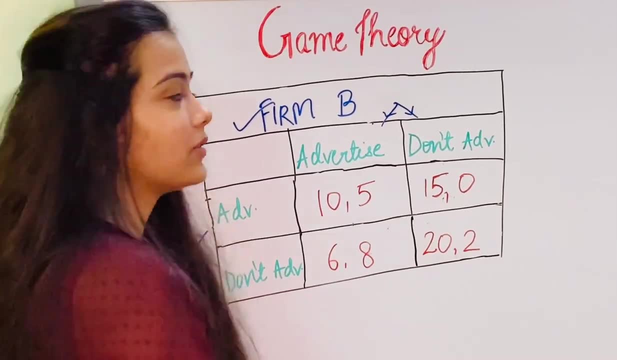 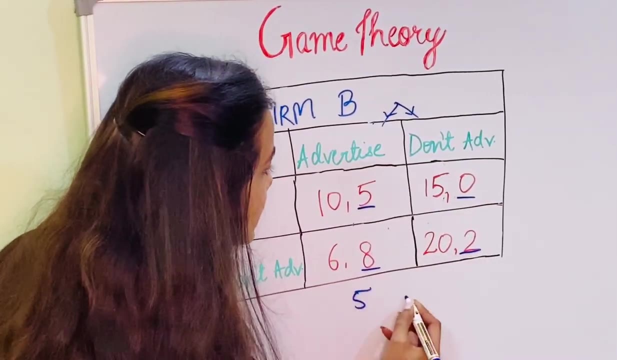 this new example, wherein we have just changed this one value. we have written 20 instead of 10 in the previous example. Now, if we consider firm B's case, we have these four values. those values five, zero, eight and two. these are similar to the values that was in the 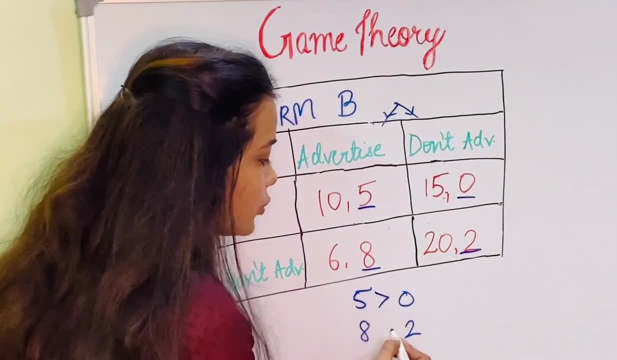 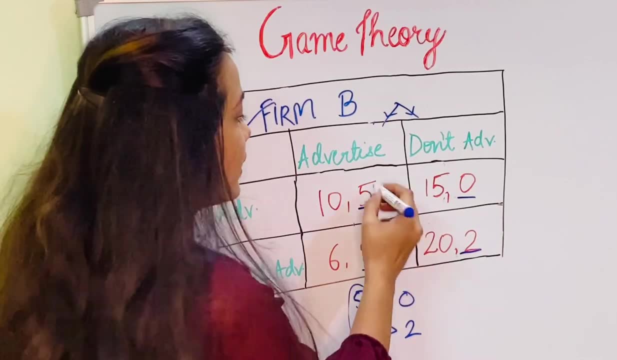 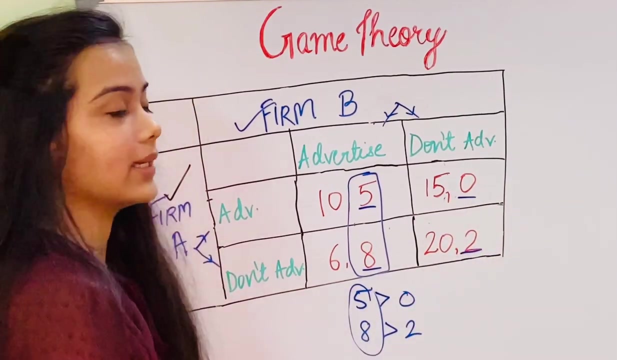 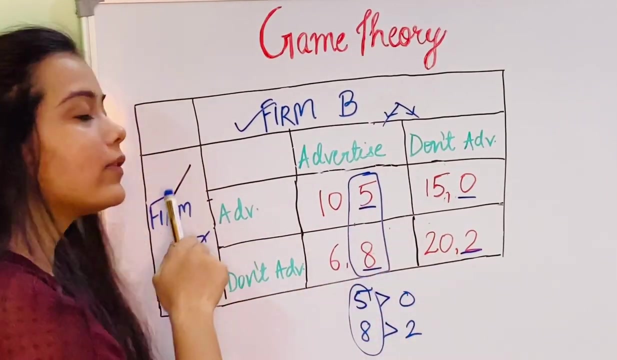 previous example. That means there are no changes again in this example also, firm B has a dominant strategy in advertising. why? because both of these values five and eight. these are greater than zero and two respectively. So firm B has a dominant strategy in advertising, provided that, whatever. 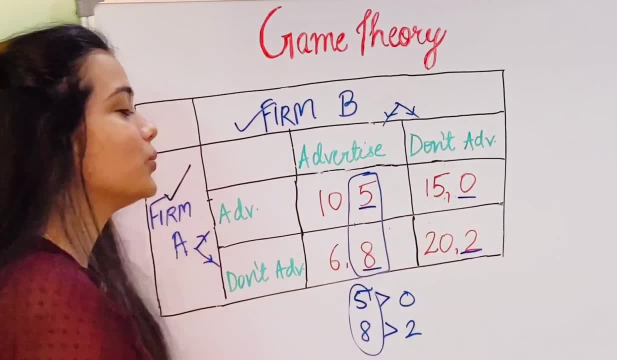 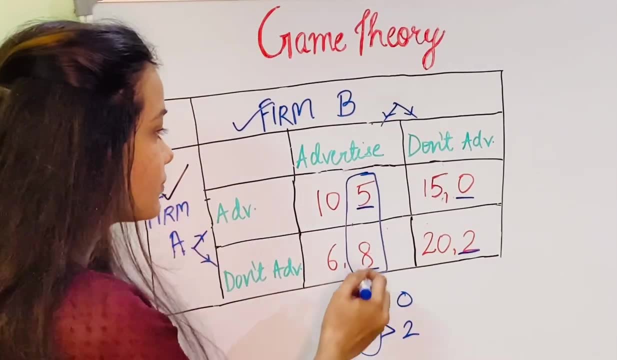 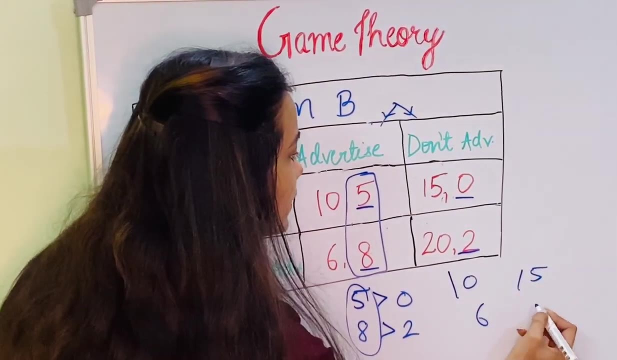 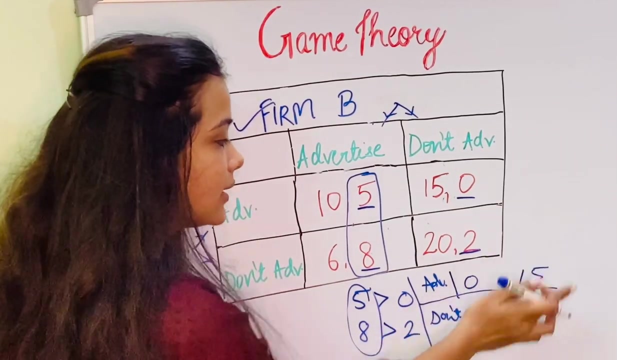 firm A does. firm B will always choose to advertise. This is firm B's case. now let us consider firm A's case. So we know that these are the payoffs of firm A. So we have these four payoffs for advertising. we have 10 and 15. 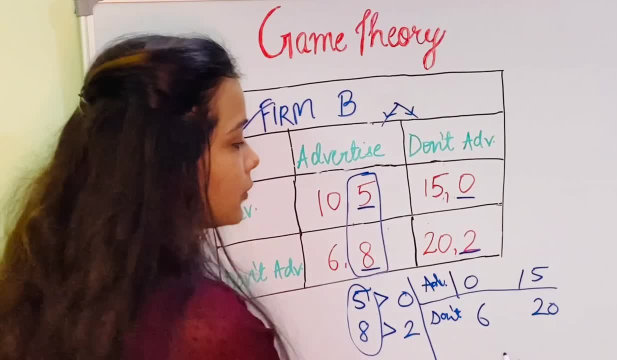 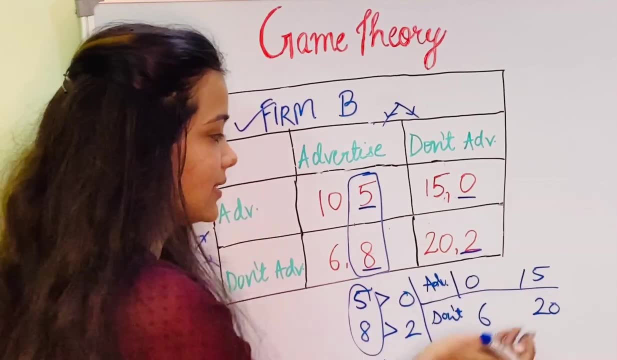 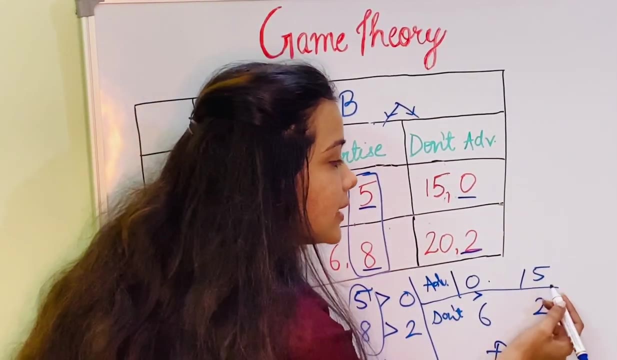 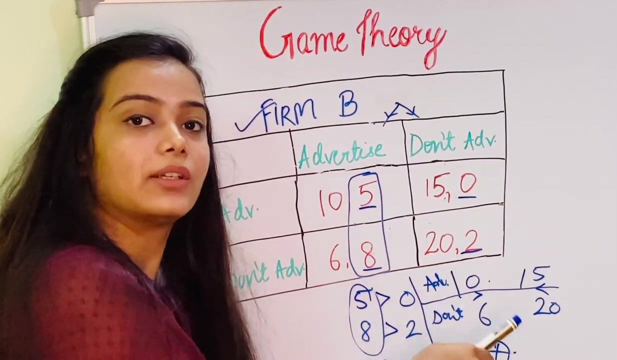 and for not advertising. we have 6 and 20 for firm A Again, if we see now we have to compare it horizontally. that is advertising versus not advertising. So 10 is greater than 6, that is fine, but 15 is not greater than 20, which means we cannot say that firm A has a dominant strategy. 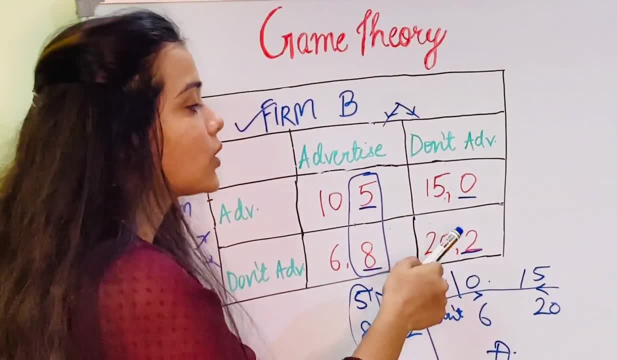 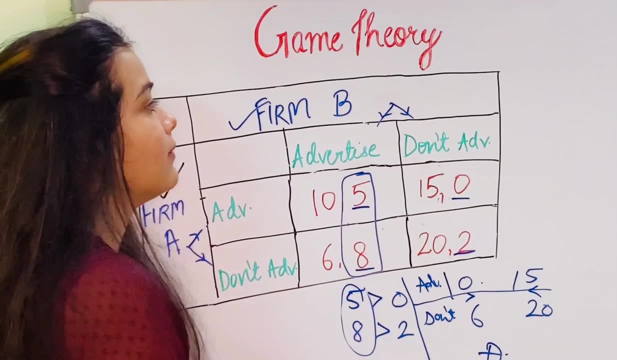 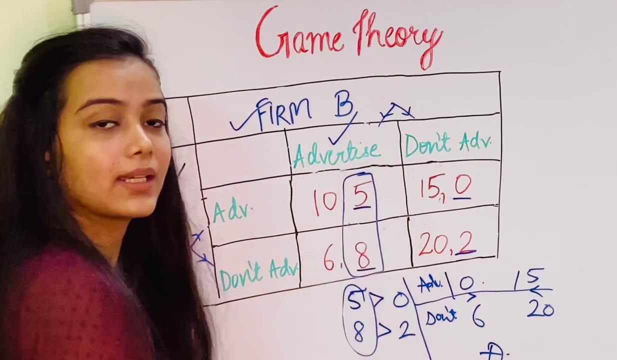 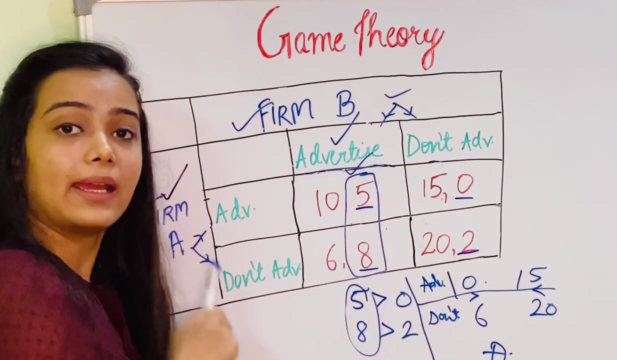 There is no one choice in which a firm would have a dominant strategy. Since firm A is not having any dominant strategy, we will move to firm B. Now firm B is choosing to advertise. firm B chooses to advertise their product. Depending on whatever firm B's decision would be, the firm that is firm A will take into consideration. 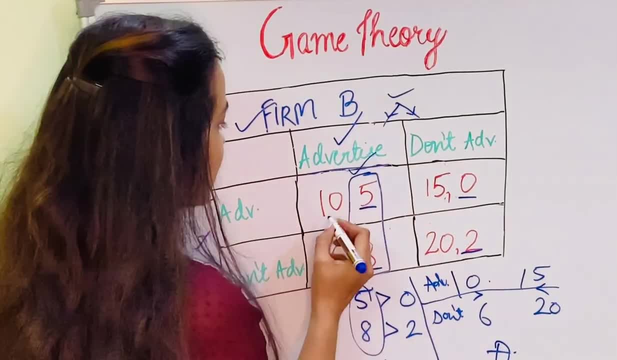 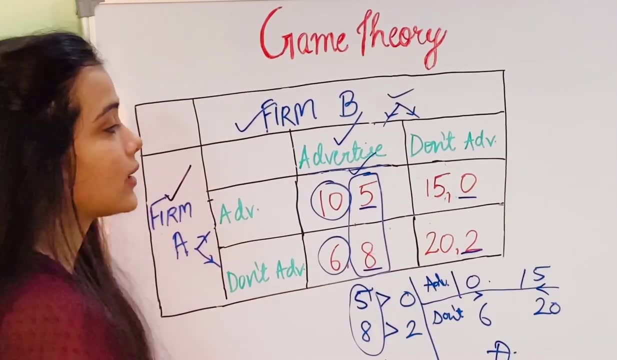 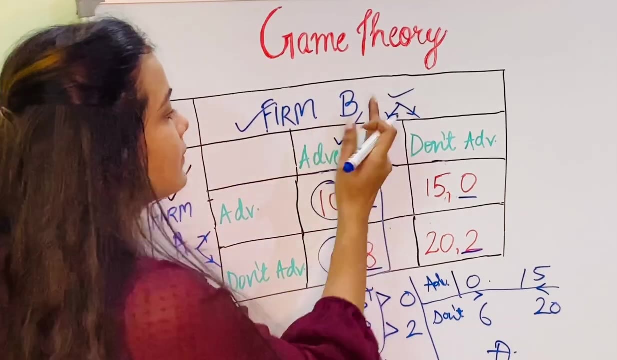 whatever firm B does. So firm B is advertising. now we'll compare firm A's payoffs, which is 10 and 6.. Now, clearly, if we have this column with us, if we have this column because firm B has a dominant strategy, We have this column because firm B will always advertise. 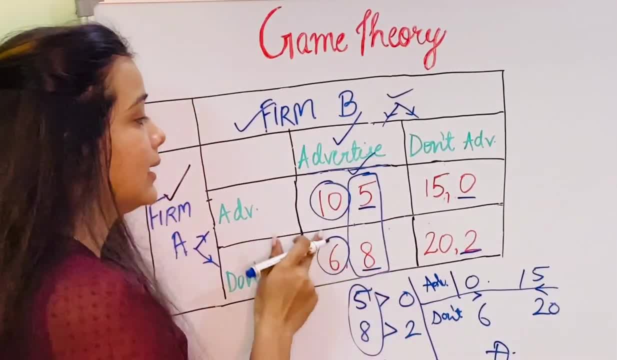 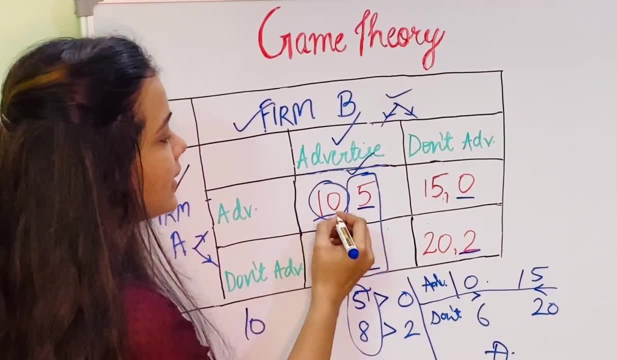 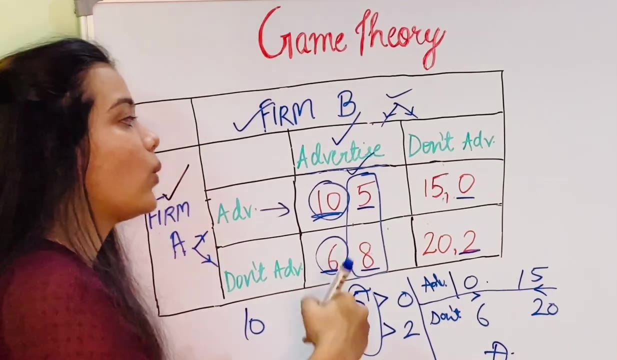 So we have this column: we have either of these two choices: Either 10 and 6. for firm A. So firm A will obviously choose 10. because 10 is greater then 6, So firm A will also choose to advertise their product, provided that firm B is also advertising. 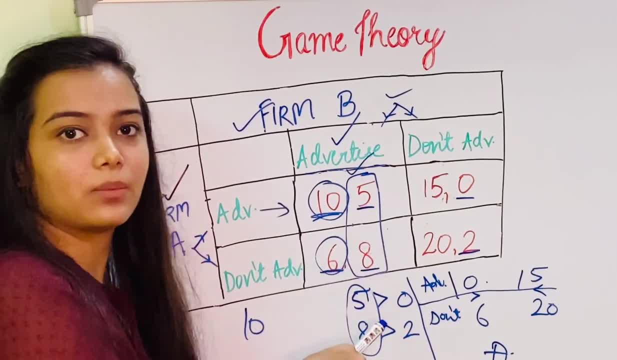 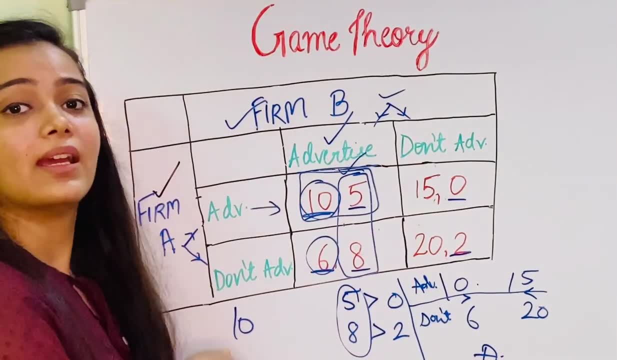 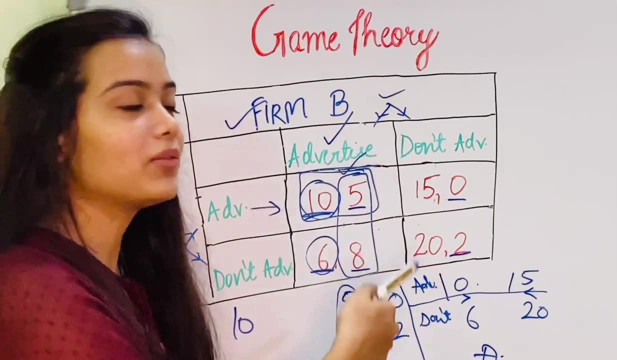 So this is wnessh equilibrium. Now, the logical outcome of this scheme is that that scheme is that both of these firms will advertise, because firm A is doing the best it can, given what firm B is doing, and firm B is also doing its best, given what firm A is doing.